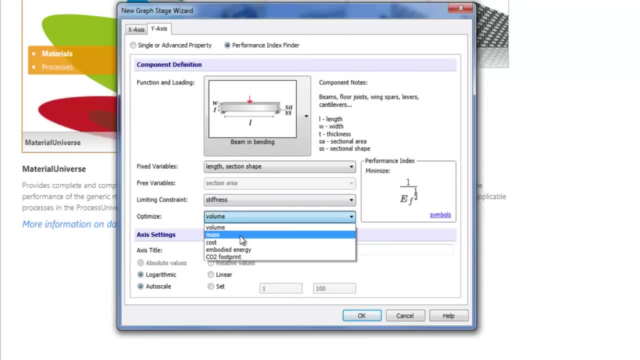 them to flex too much in use and we want to minimise mass. This tells us that for a light, stiff beam in bending we need to select materials with a low value of density divided by the square root of flexural modulus. Having looked at weight, we repeat the process. 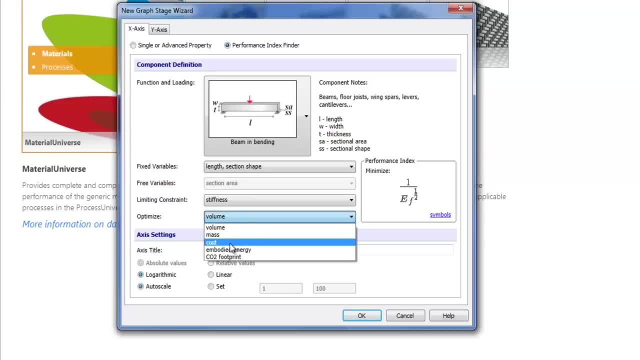 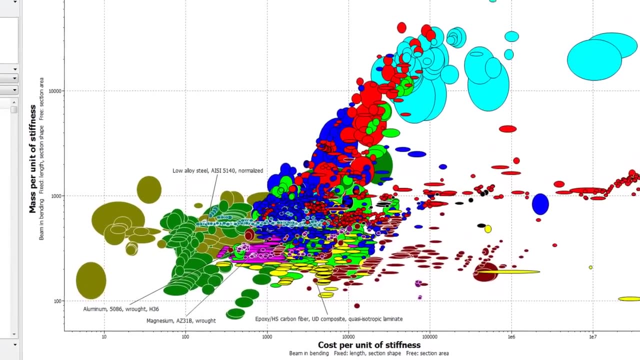 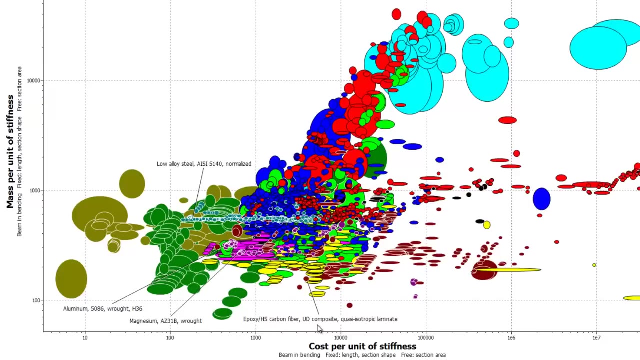 for cost on the x-axis, which updates the material index to incorporate cost per kilogram. This creates a mass vs cost trade-off plot for all materials, with optimal candidates appearing in the bottom left-hand corner. However, we also need to consider some other essential design requirements and add in constraints. 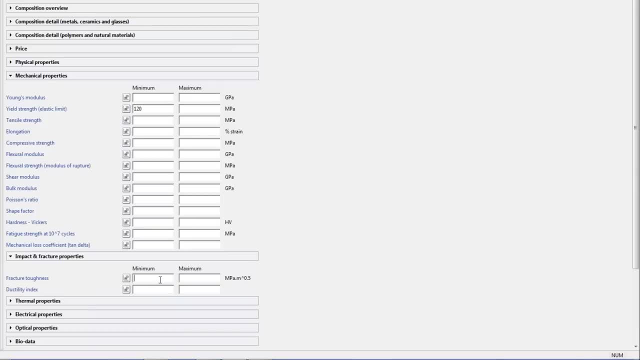 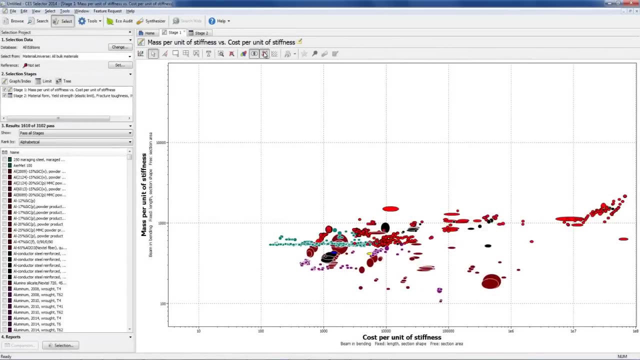 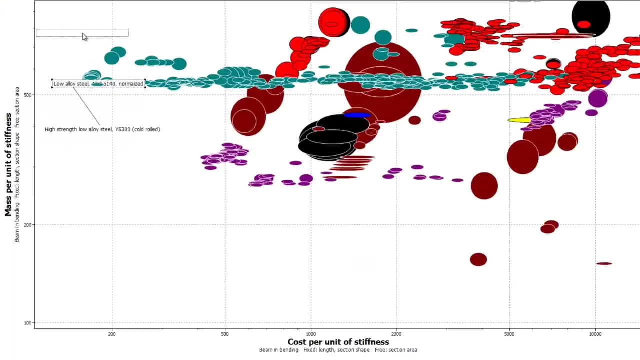 on strength, toughness and durability. This eliminates all materials that don't meet these requirements, leaving us with a mass versus cost trade-off for the remaining viable materials. Low alloy steels are lowest cost, but relatively heavy. carbon fibre composites are much lighter. 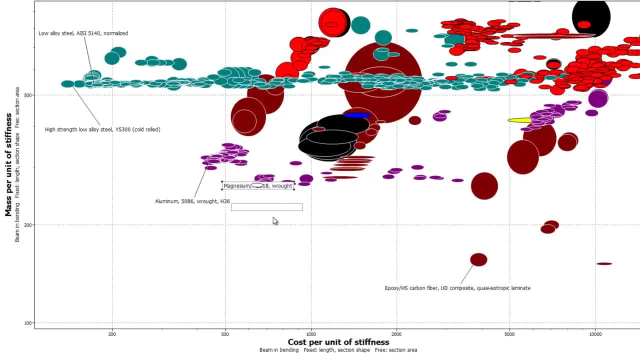 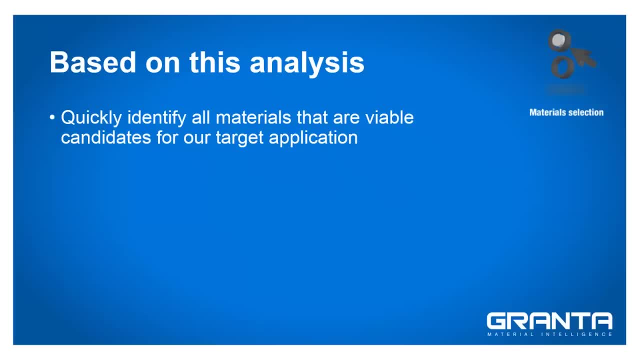 but expensive. aluminium and magnesium alloys fall between the two. Based on this analysis, we can quickly identify all materials that are viable candidates for our target application, investigate and understand the cost versus mass trade-off associated with the different material options and readily communicate the reasons for our material choice. 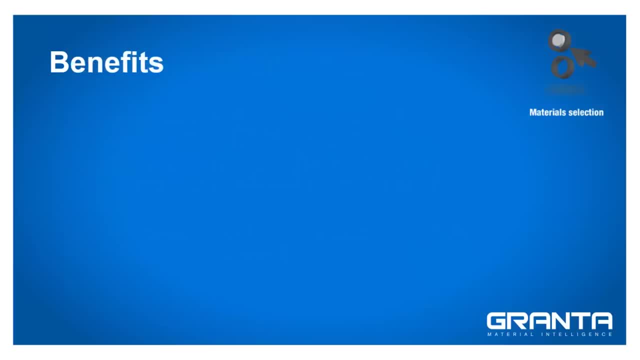 to project sponsors. With such an approach, we can build confidence in our material choices, focus our development on the most appropriate materials, reduce prototyping and testing iterations and reduce our time to market. If you have further questions or are interested in purchasing CS Selector, please contact. 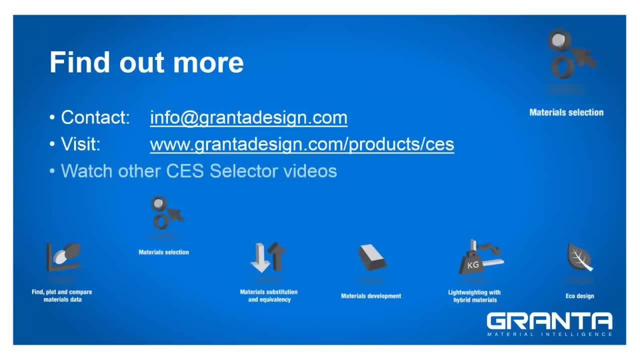 us directly explore our website or watch other videos demonstrating further applications of CS Selector.